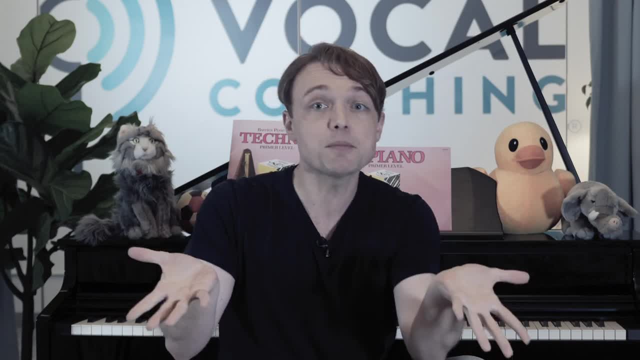 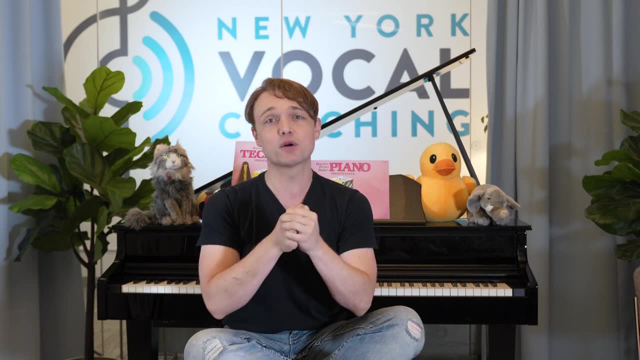 cough, never yell, never whisper, never do a glottal, never be breathy, never lift your larynx, never sing into your nose, and the list goes on. And I get it, I get it. It's terrifying for a voice teacher to think they might somehow hurt a child's voice, But let 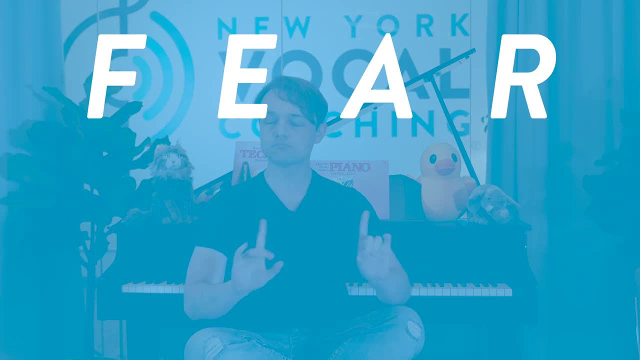 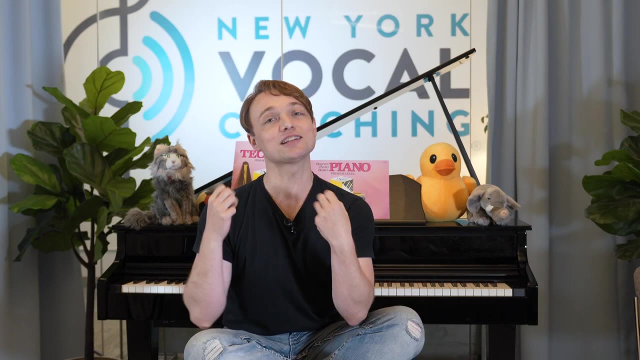 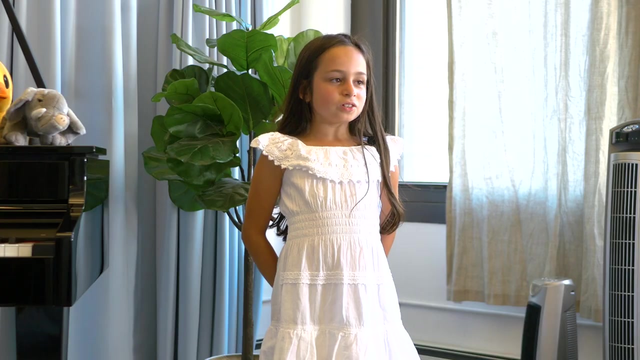 me submit this to you as we get started: Fear never inspires, Love always inspires. And children just love to sing. I love to sing, You sure do? I love to sing. Good now, I love Swedish Fish. You cannot sing that. 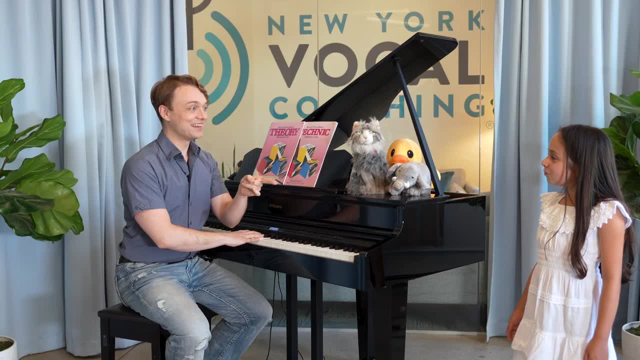 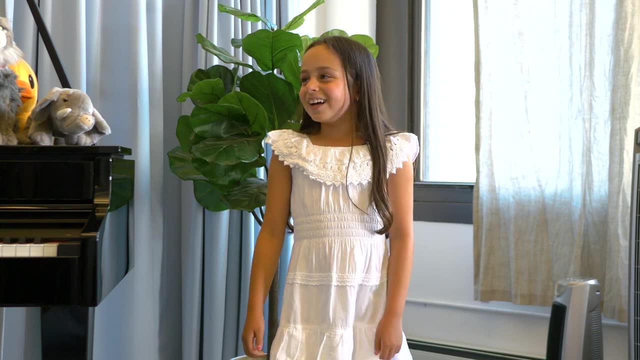 Yeah, you can, I can sing. It's hard to even say the word Swedish Fish. Try it, I love Swedish Fish. Yes, you did, I love Swedish Fish. Good, now I love to sing. I love to sing. 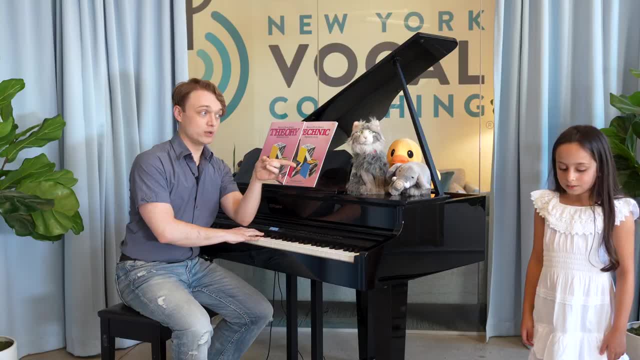 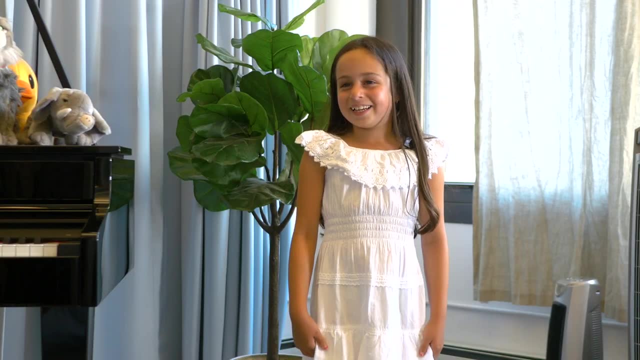 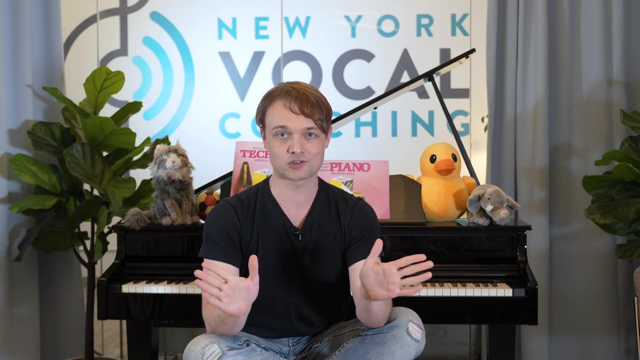 Yeah, I love to sing. Swedish Fish. I love Swedish Fish. Good, I love to sing. I love to sing, Yes, you do, And they'll be singing and whispering and yelling and drinking. They'll be drinking hot and cold drinks, with us or without us. so isn't it far better for? 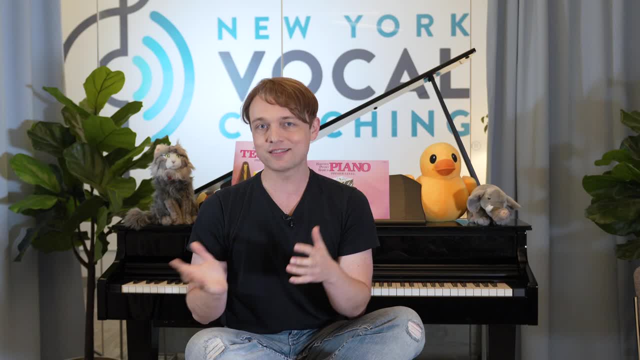 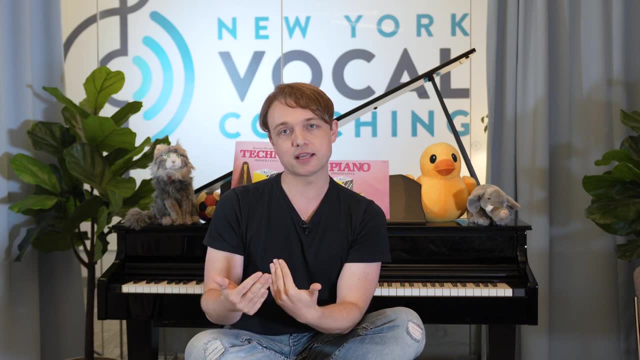 them to be in the trusted care of a vocal professional than to have to figure it out all by themselves. The answer is pretty clear. So we don't need to be fearful about teaching kids. We just need to be patient, caring and wise. 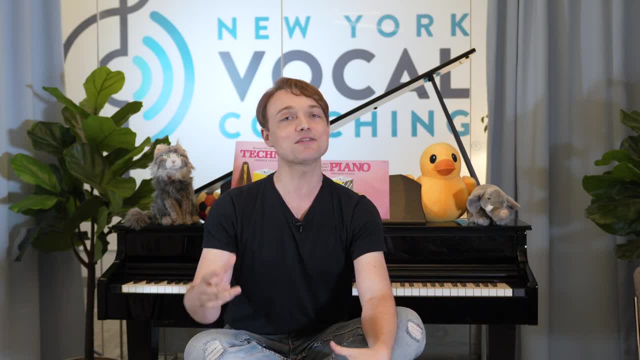 And that starts with understanding how a child's voice is different from an adult's voice. Now, there are some things that we don't need to be careful about when we're teaching kids. One of the things that we need to be careful about when we're teaching kids is that we need 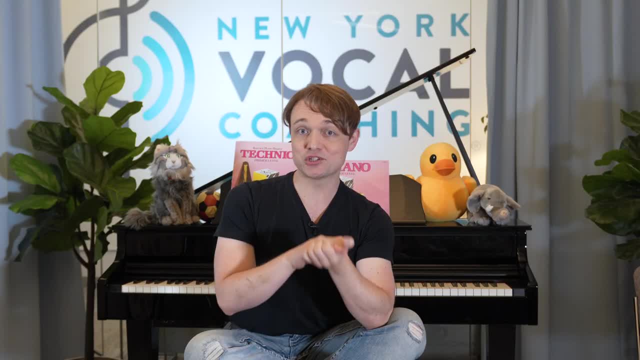 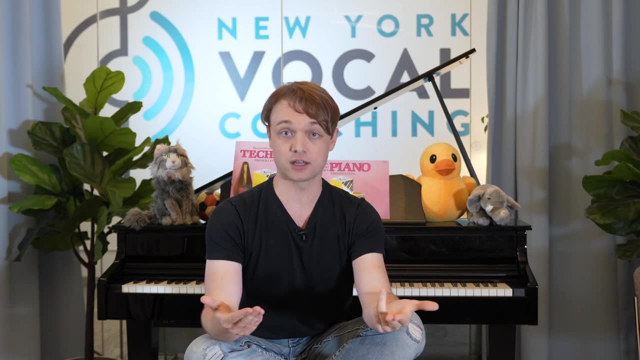 to be patient, caring and wise, And that starts with understanding how a child's voice is different from an adult's voice. Now, there are some important differences in children that we want to understand. Basically, it comes down to size and development of things like the lungs. 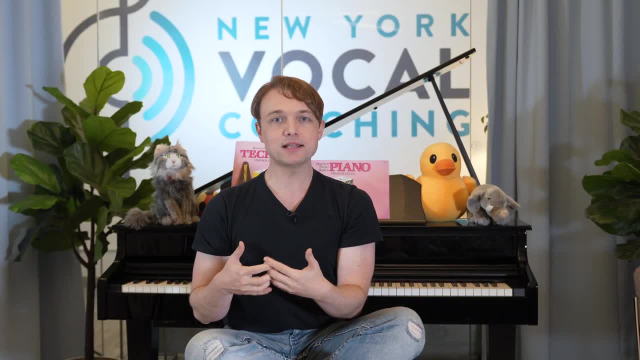 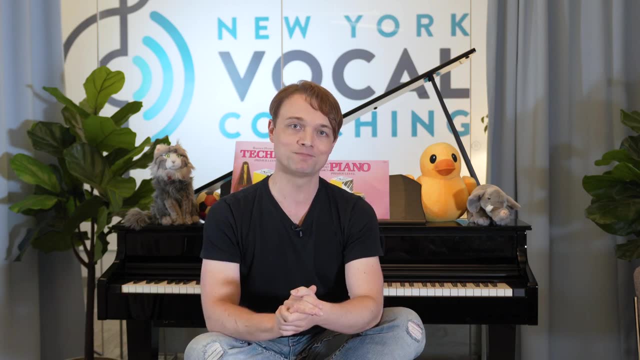 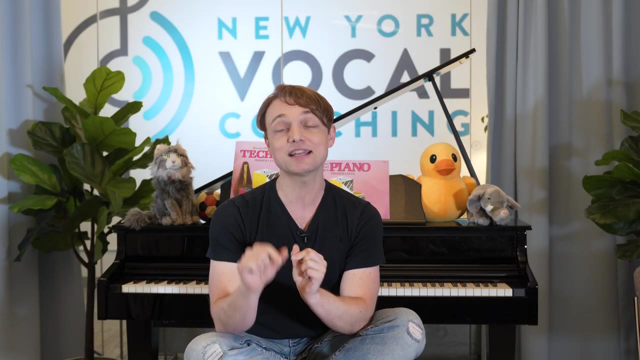 The lungs are smaller and less developed in children. That means, for example, they won't be able to sustain notes as long as adults And we won't expect them to The vocal folds. The vocal folds are smaller in children than adults and layers like the intermediate and 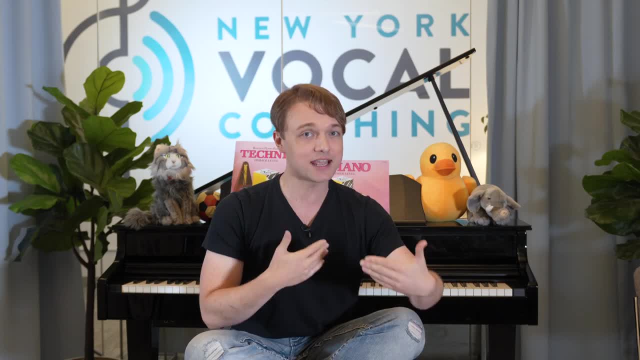 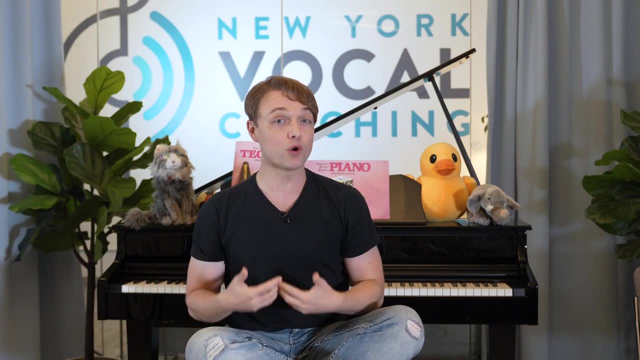 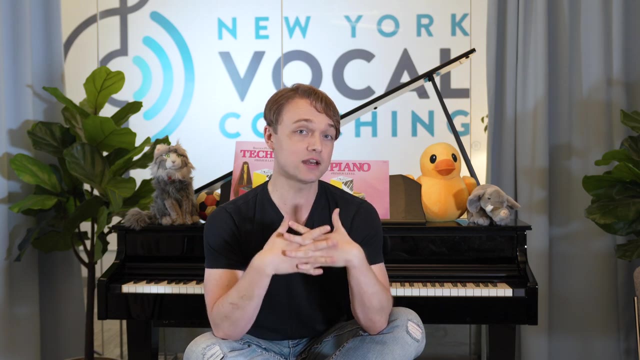 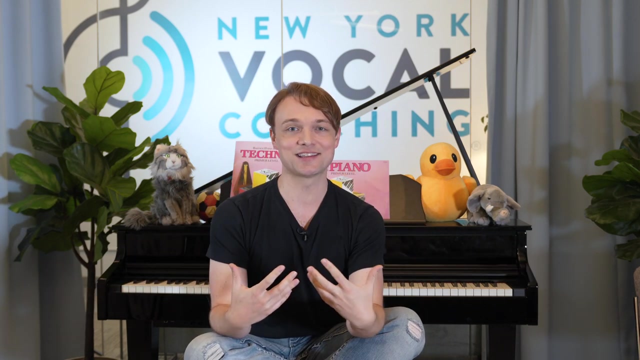 deep lamina propria don't fully develop. This consideration impacts how aggressive we are in pursuing fast results with vocal registration. What about resonance? The resonance of a child's voice is different than an adult's. Simply put, children sound brighter. They have higher, brighter formants. 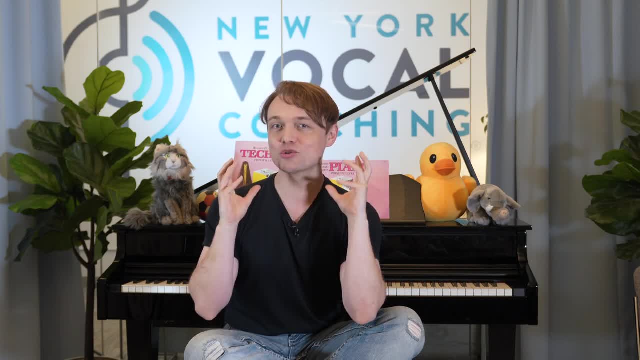 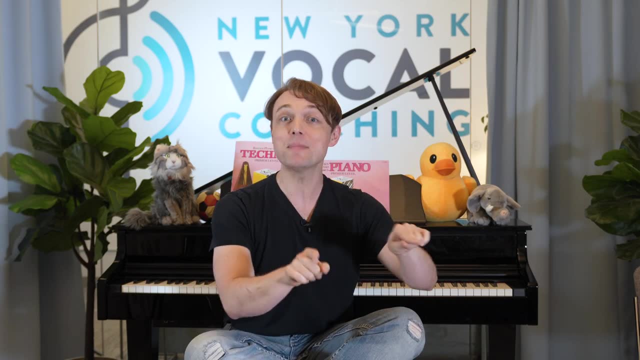 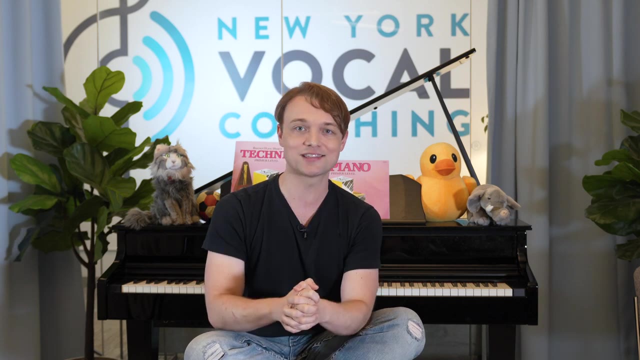 This has to do with the larynx sitting a little bit higher and also the smaller spaces in the pharynx mouth and nasolabium. That's what we're looking for. Remember, smaller spaces make brighter sounds. This affects our expectations as far as tone quality when working with kids. 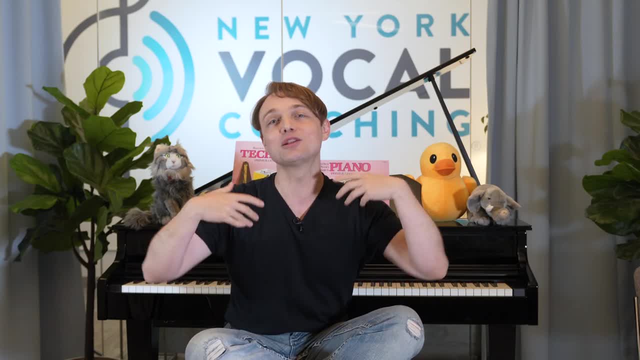 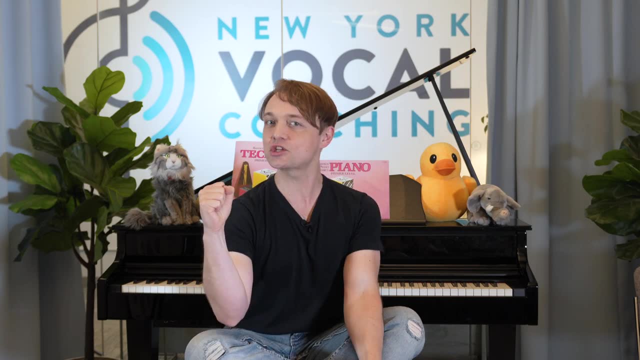 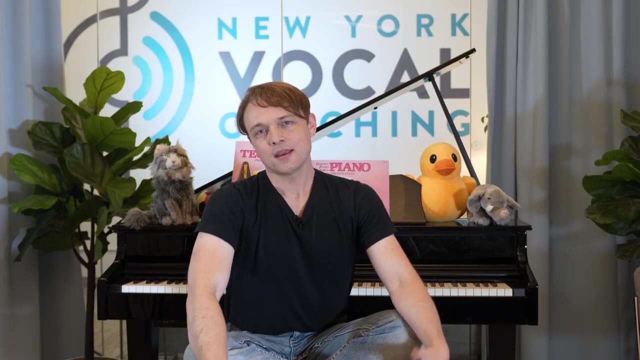 In other words, it's okay to let them be a little brighter than an adult. Okay, now that we've explored some of the key differences, let's get to work on some vocal exercises. Vocal exercises: Same way, we have youth sports like little league soccer, gymnastics. we have little. 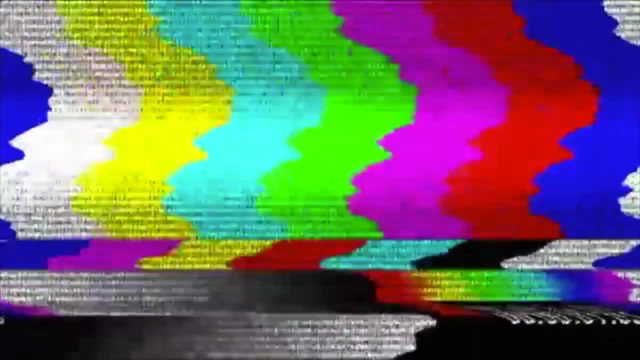 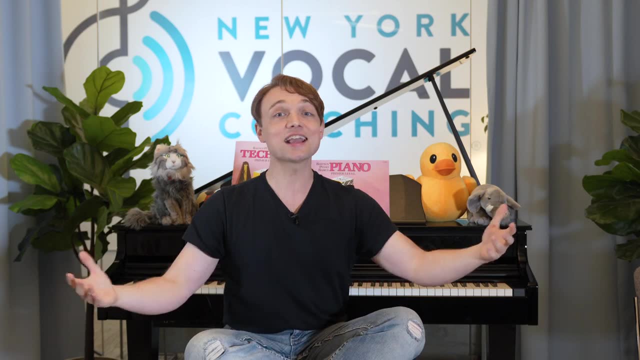 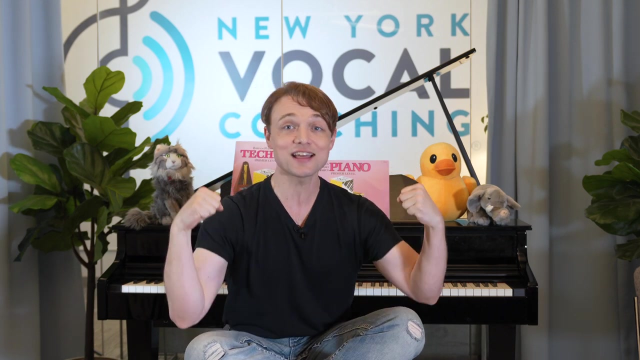 singing athletes. Sports allow kids to challenge themselves, while we monitor their development in responsible ways. Singing is no different. We can help young singers to develop good habits and coordinations with their vocal athleticism. We want our exercises to be fun and simple, but still focused on a specific goal. 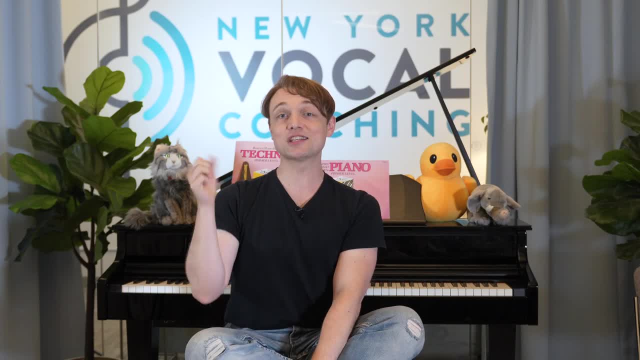 We want our exercises to be fun and simple, but still focused on a specific goal. We want our exercises to be fun and simple, but still focused on a specific goal. For example, this little woo-hoo celebration exercise encourages a positive spirit and 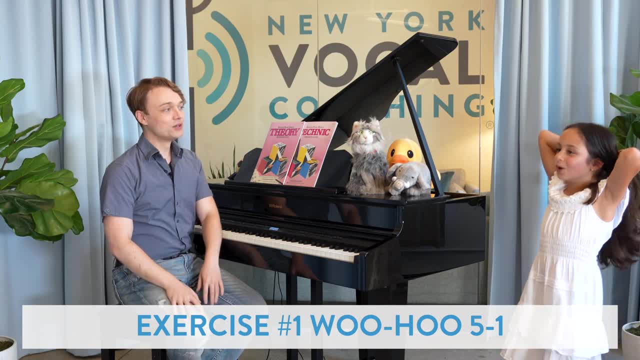 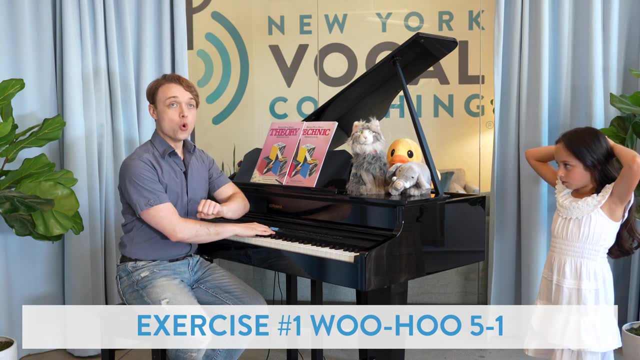 helps stretch the vocal folds. Woo-hoo, Good. And can you do one of these? Woo-hoo, Woo-hoo Good. How about this? Woo-hoo, Woo-hoo, Woo-hoo, Woo-hoo, Yeah. 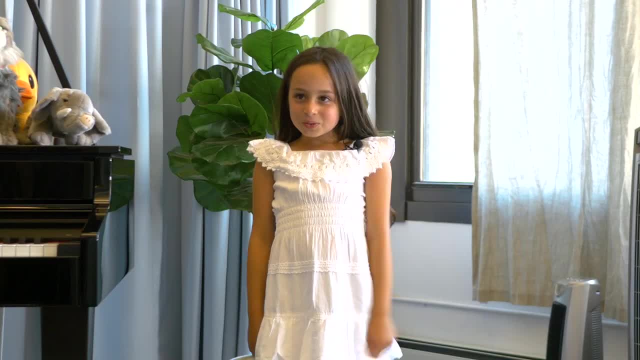 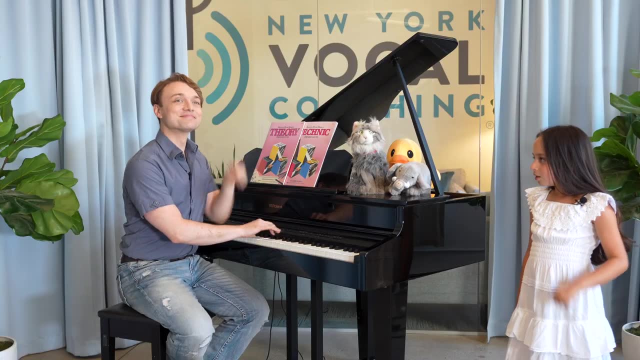 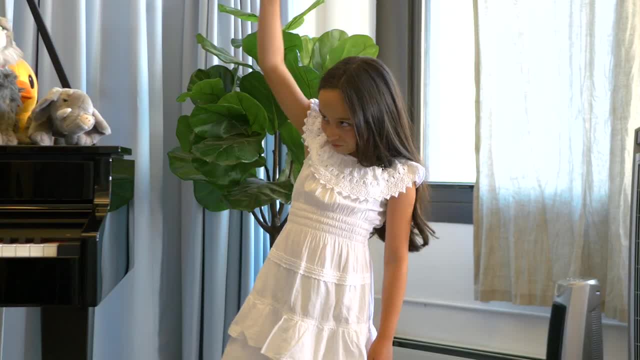 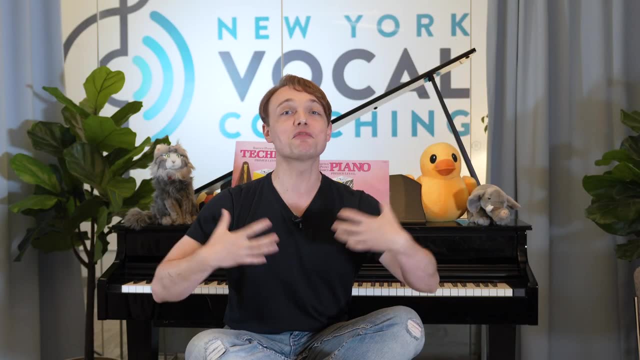 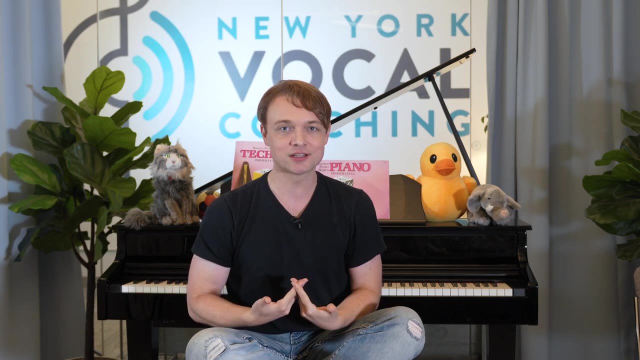 Good Now, Swedish Fish. Swedish Fish 먹어. Good Now. woo-hoo, Woo-hoo, Yeah. The next exercise brings in a spirit of play. It personalizes and physicalizes the sound making. It helps to develop chest voice. 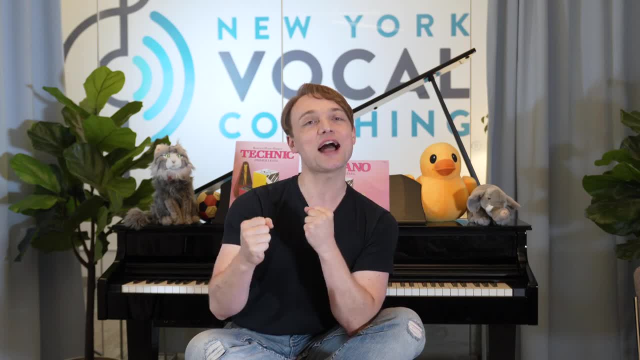 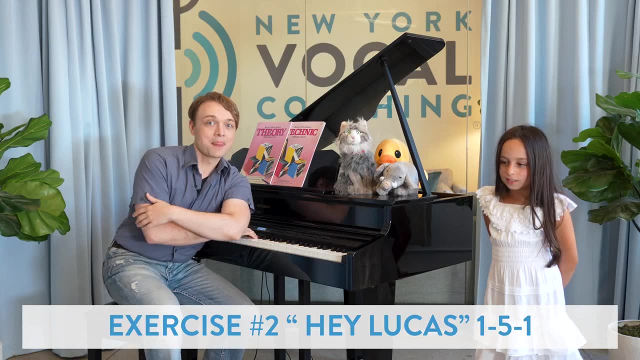 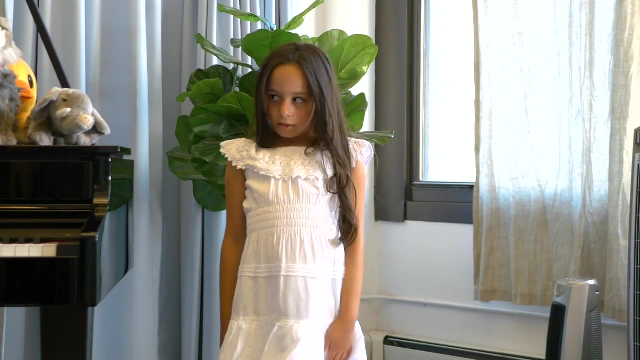 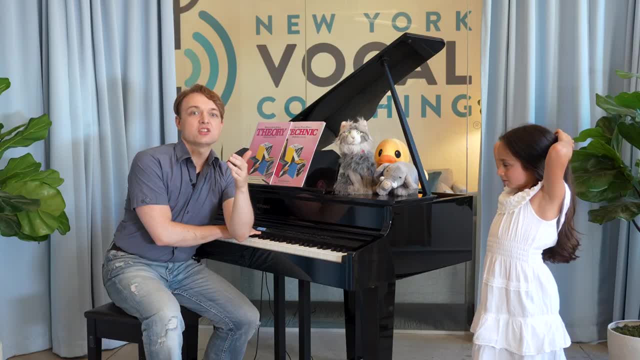 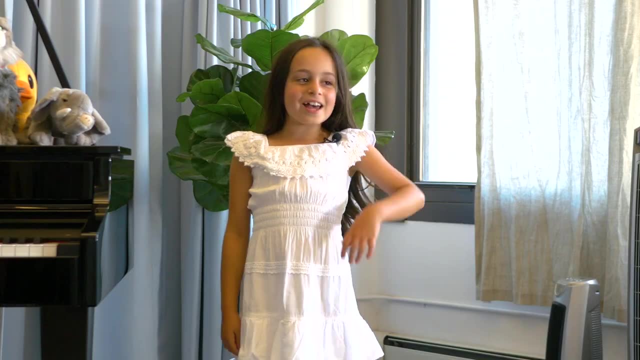 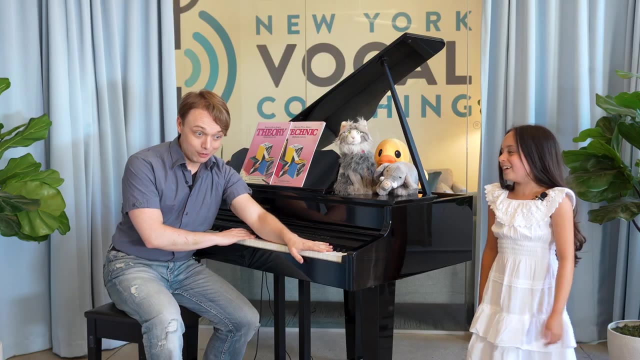 Yeah, Skittle gummies, Hey, Skittle gummies, Hey, Skittle gummies. Hey Lucas, Hey Lucas, Hey Lucas. Uh-huh, Hey Lucas. Right, Hey Lucas. Okay, I don't know about that now. All right, let's go back. 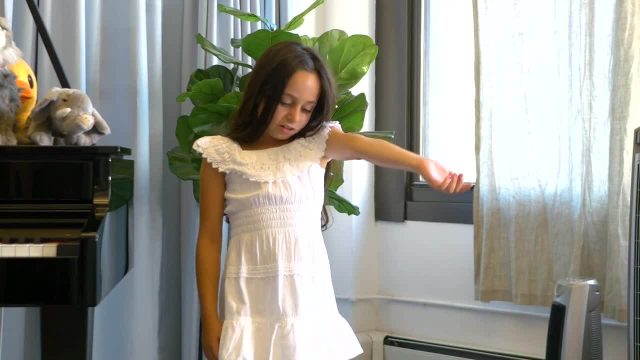 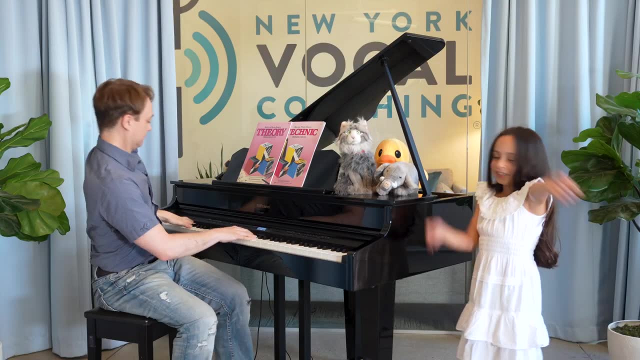 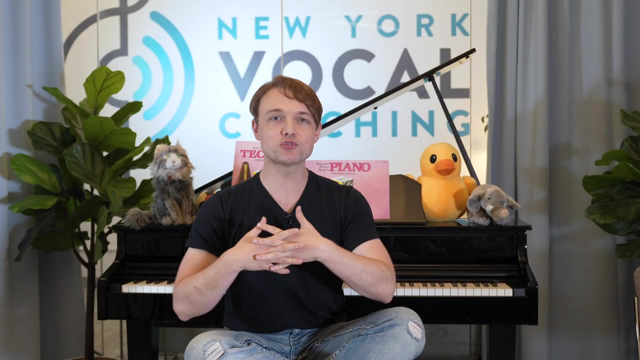 Hey Lucas, Uh-huh, Two more. Hey Lucas, Uh-huh, uh-huh, Hey Lucas, Yeah, yeah, yeah. Hey Lucas Done Whoo good job. Next we'll use a prop and some creativity for an exercise that builds the mix by encouraging. 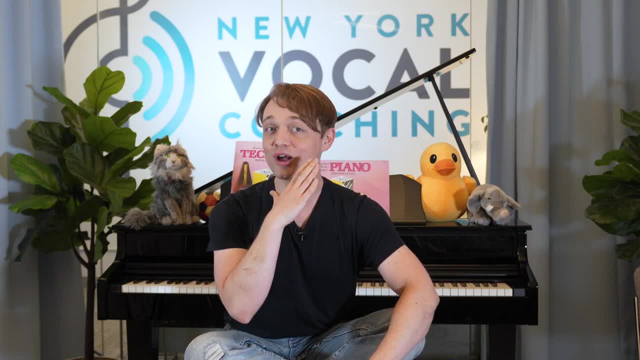 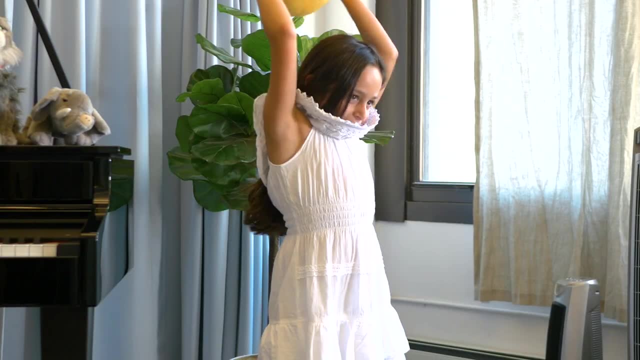 a narrow opening. The music is called. it's a little ambusher, a free forward tongue and also twang: Quack, quack, quack, quack, quack. Yeah, okay. Quack, quack, quack, quack, quack quack. Whoa, That's a quack attack right there. Okay, Quack, quack, quack, quack, quack, quack. A little too violent. Okay, Let's go back. I want you to be. let's have a nice ducky. 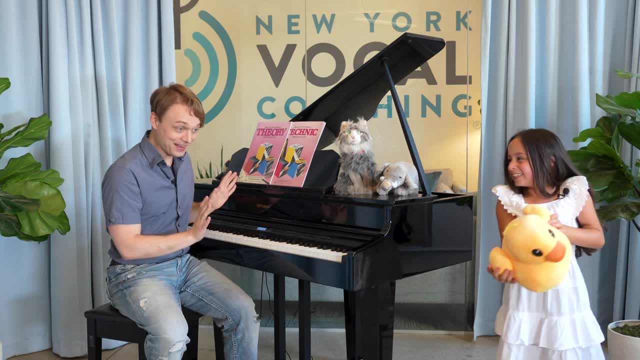 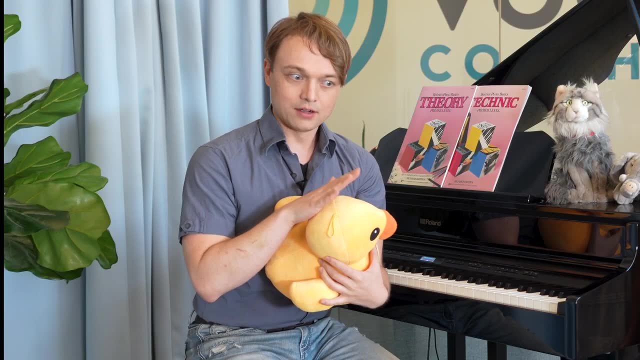 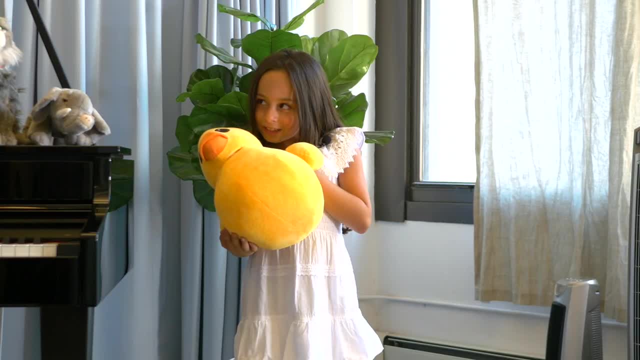 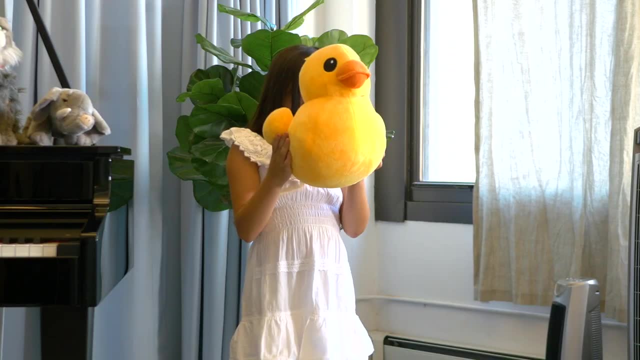 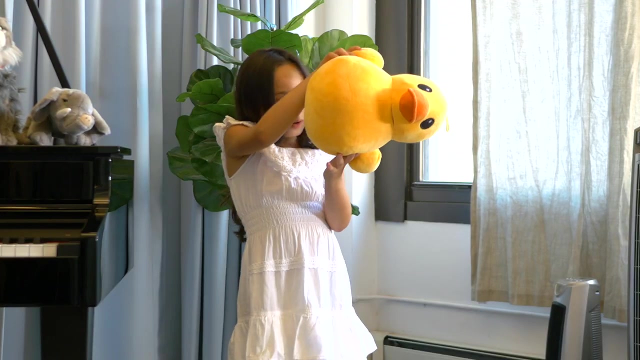 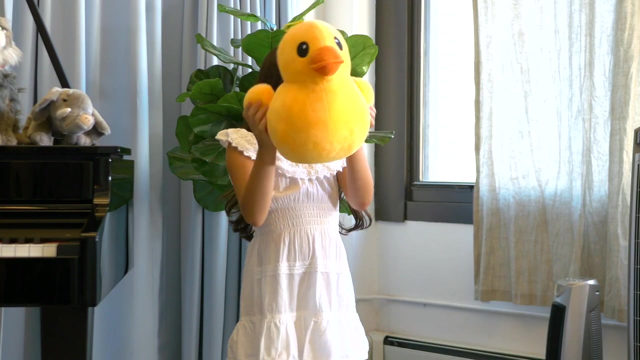 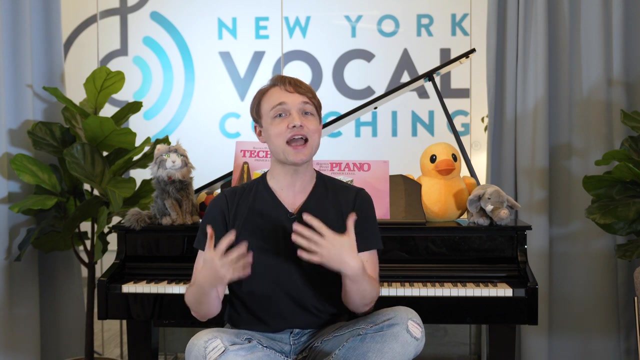 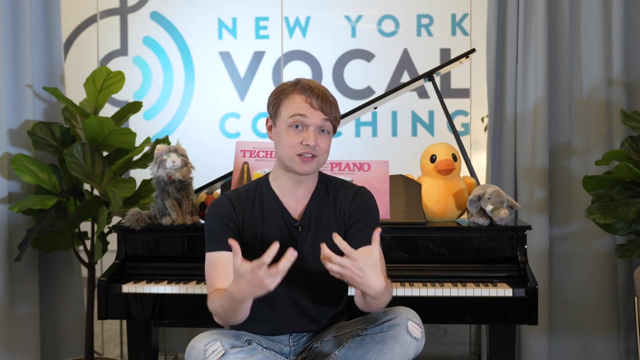 Quack, Quack, Quack friend, nice quack friend". There are literally hundreds more examples, but I hope these give you a a general sense of exercises that are engaging and specific. But building a young singer is about more than exercising their voice. 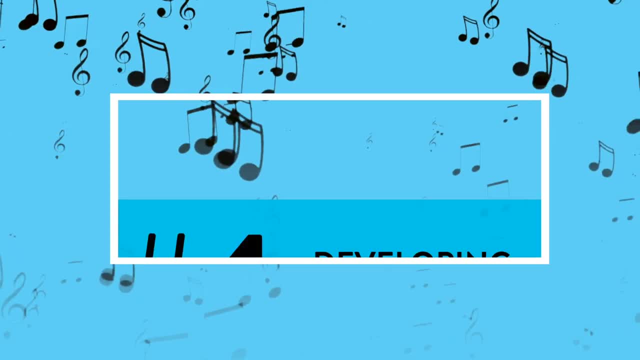 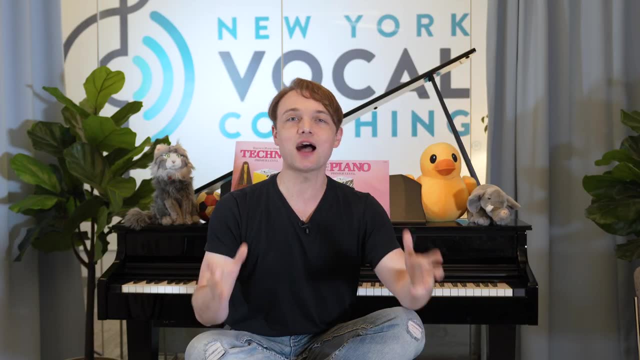 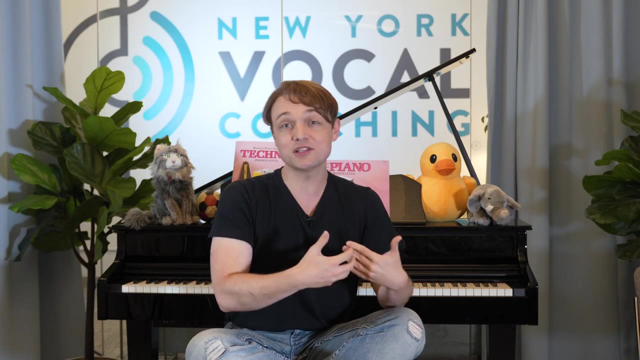 We also want to develop musicianship. One of the best parts of working with children is they have the gift of time So many years ahead to master their craft, So it's important to make sure they develop into good singers, but also good musicians. 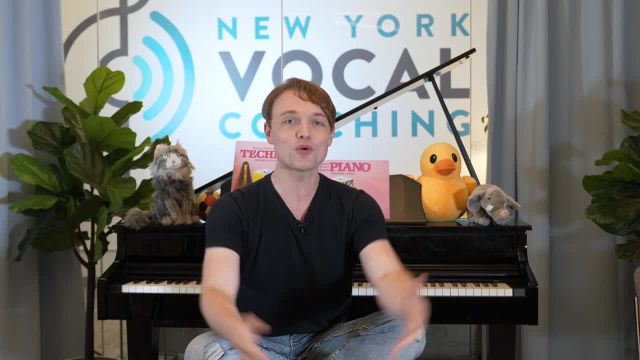 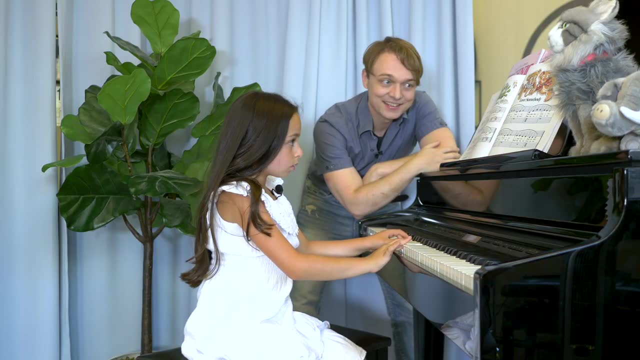 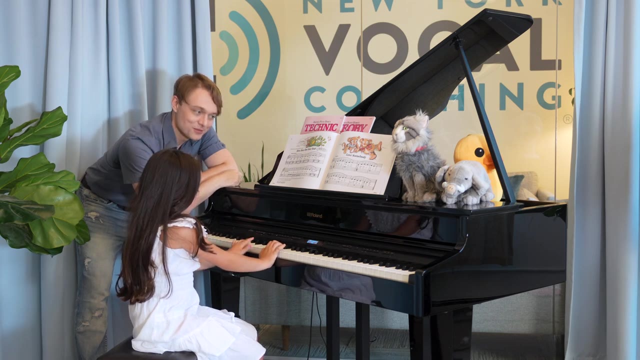 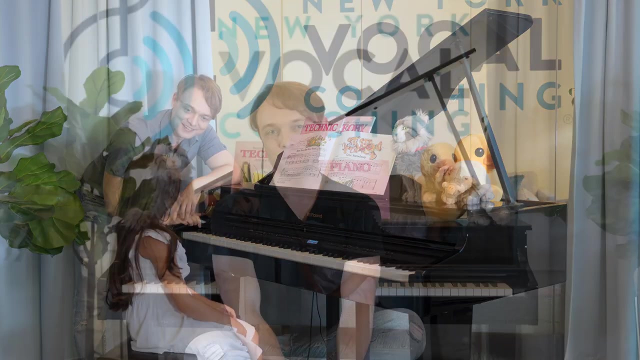 In the case of Emi, we throw some piano training in with her voice lessons. Okay, Yeah, Yeah, good job, that was it, you did it. If you can't add instruments to the lessons, you might explore adding some creative music. 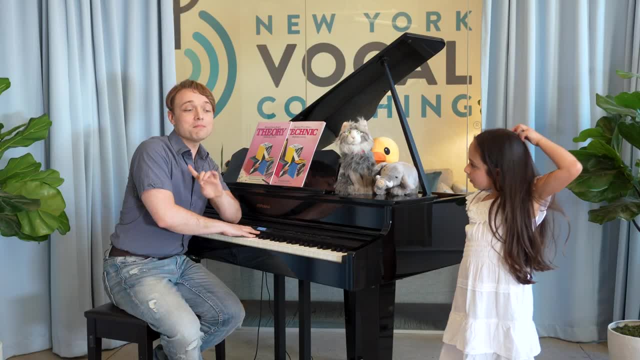 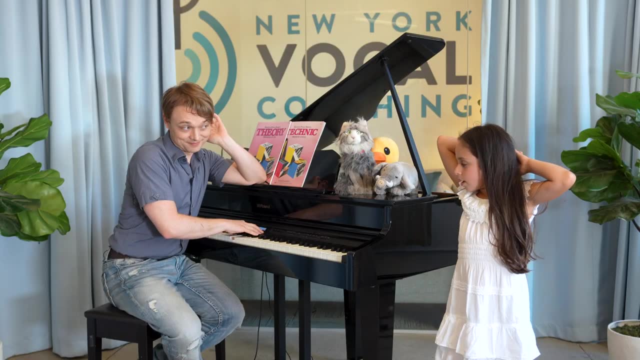 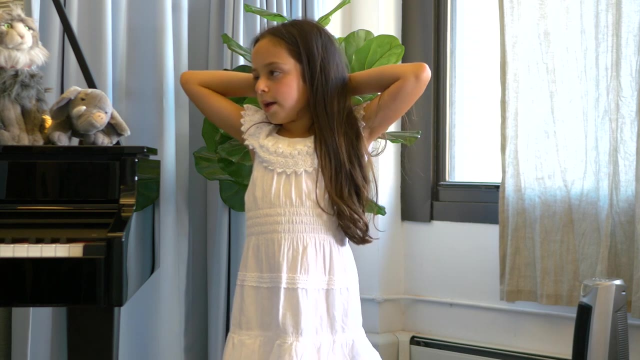 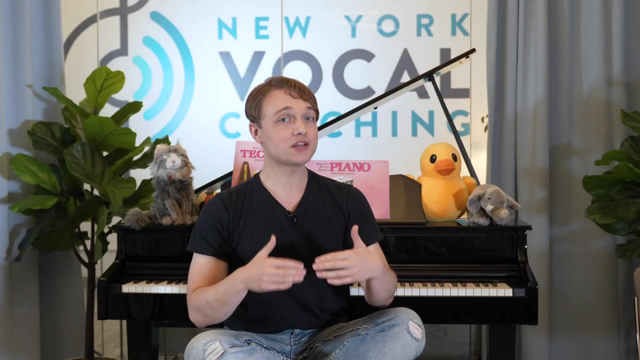 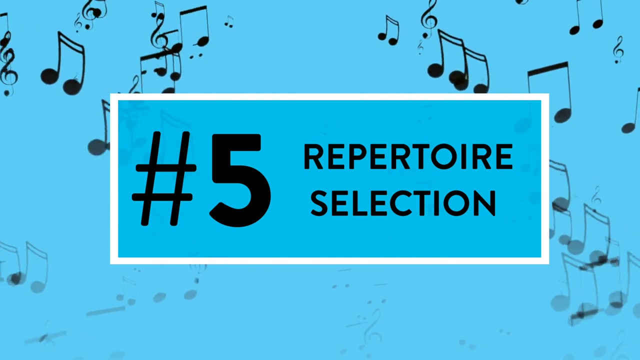 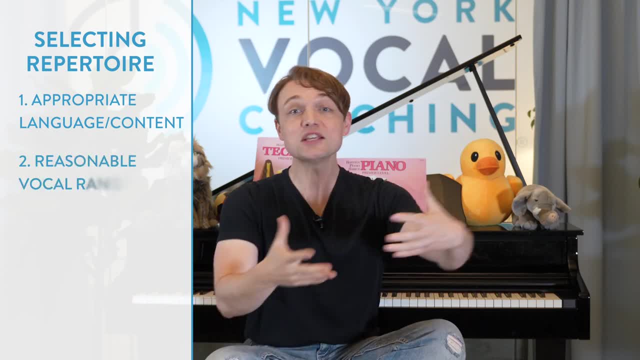 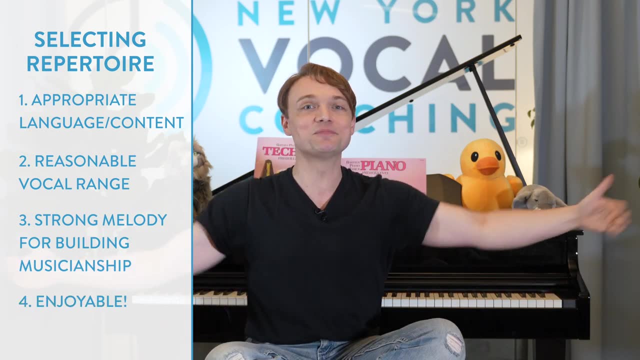 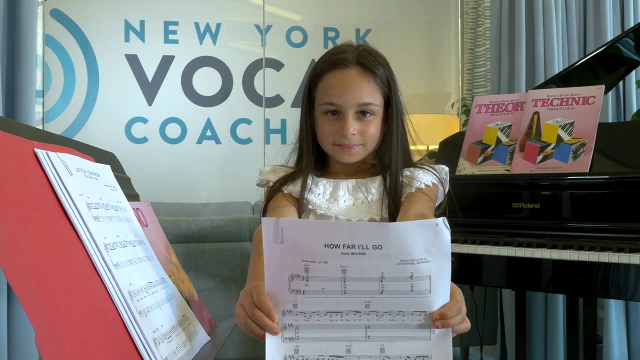 Appropriate language and content, reasonable vocal range, a strong melody for building musicianship and it's enjoyable. My recommendation is to start with enjoyable, something that the singer absolutely loves. This guarantees that they're going to have a good time. If the content is appropriate, then we're good to go. 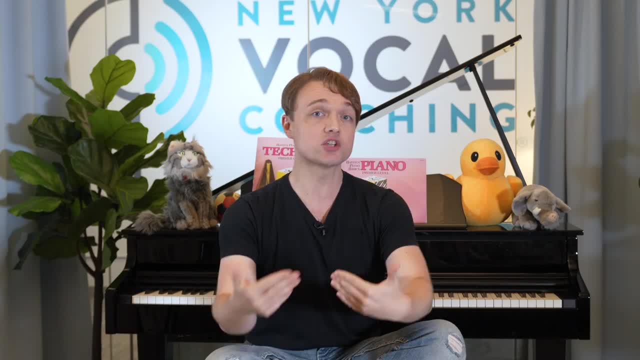 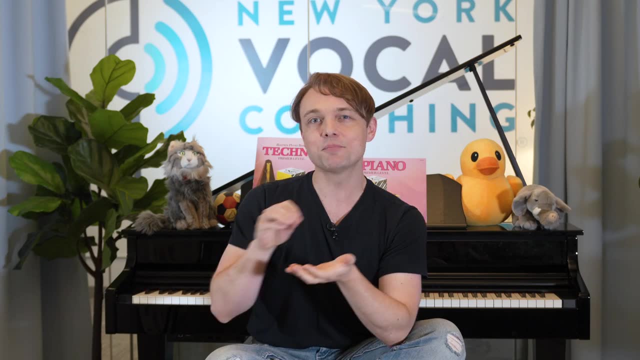 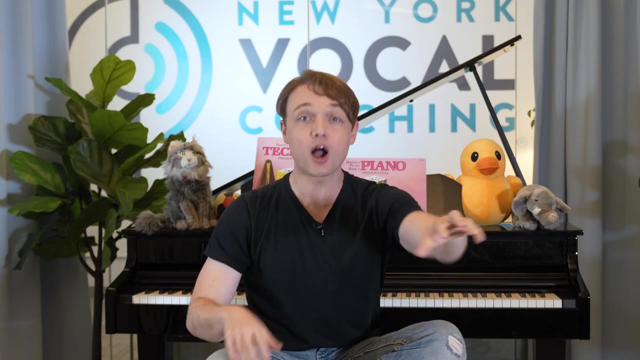 If the vocal range is too high or too low, you can always adjust the key. And as for melody, remember you can always recommend another song later on. But it's important to start with the child's interest. Try to work with that for a while and then branch out to other repertoire once they're loving the lessons. 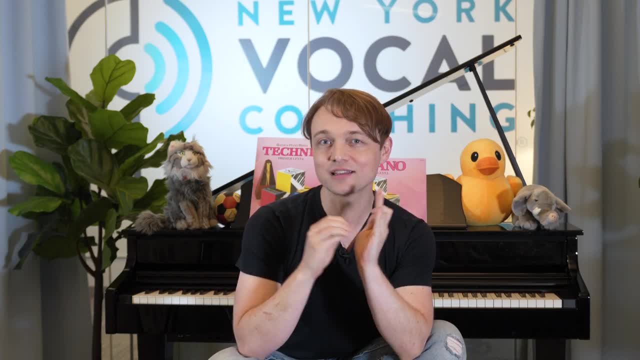 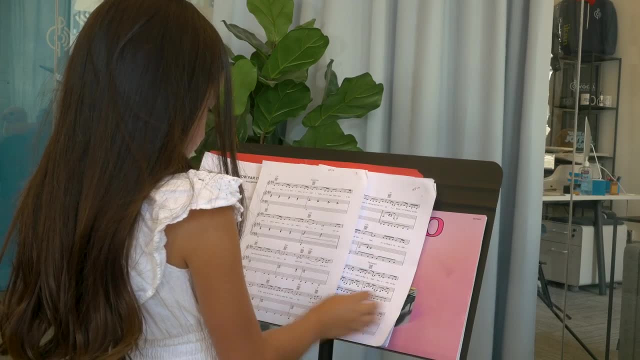 One important thing though: even with a song they love, make sure they've got the sheet music right in front of them. They might say, but I can't read music. Well, not yet, But this is a way to start. 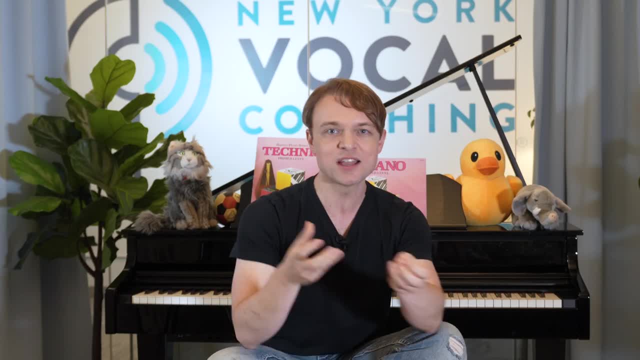 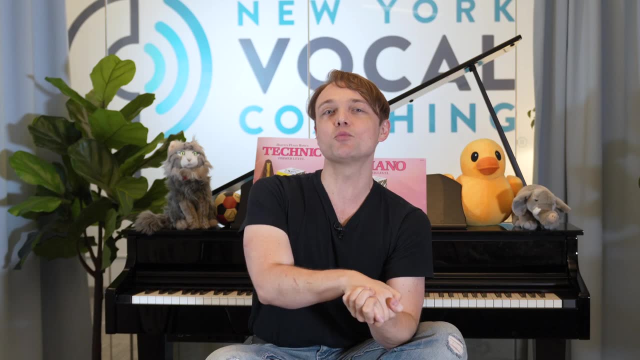 By seeing the contour of the line, the notes, the rhythms, the symbols, we can learn a lot In a moment. Emmy is going to sing a song for us, But first here are some ways to go deeper on your singing or teaching journey. 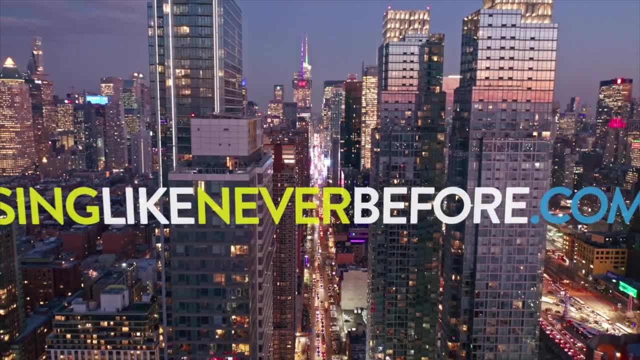 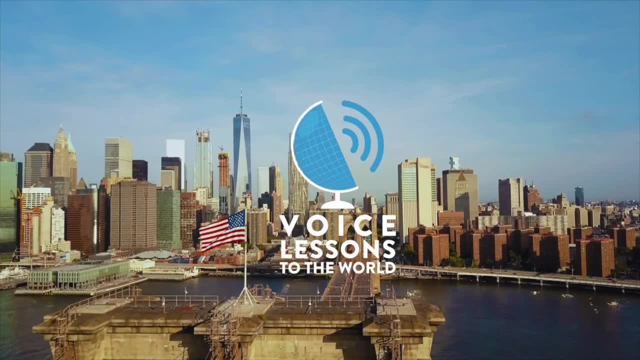 To get your copy of Justin Stoney's book Sing Like Never Before, visit singlikeneverbeforecom. If you'd like a vocal course that you can do from home, check out the Voice Lessons to the World vocal course. Our 12-part program takes you on a journey from beginner to master level vocal exercises. 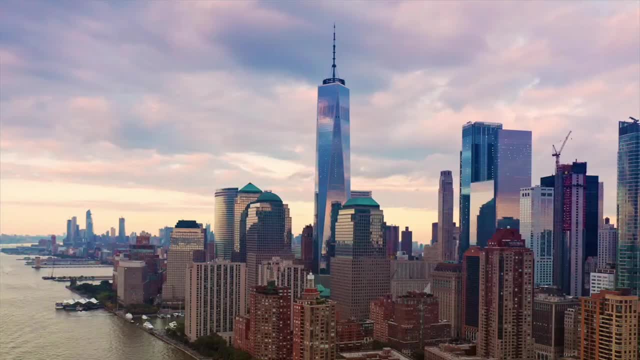 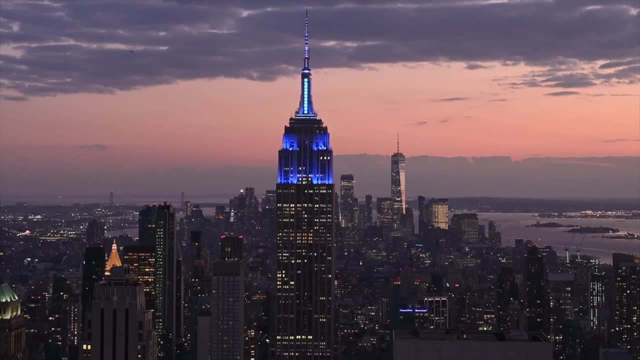 Find it at voicelessonstotheworldcom For voice lessons with the NYVC staff. please visit newyorkvocalcoachingcom. If you're a voice teacher looking to master your craft, join our worldwide community at voiceteachertrainingcom. 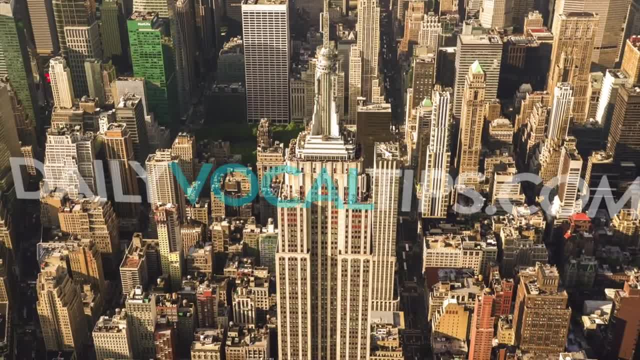 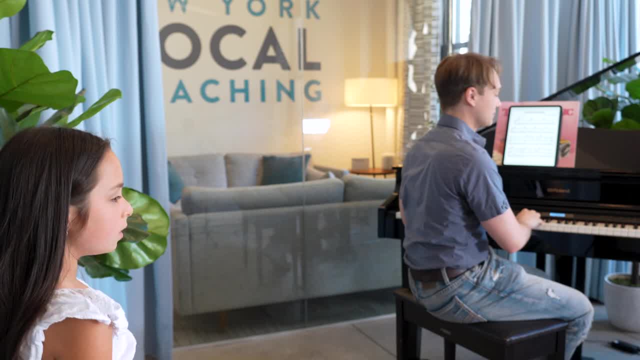 Finally, if you'd like free vocal tips sent to you each day, sign up at dailyvocaltipscom And don't forget to subscribe to our channel for more videos like this. Thanks for watching. Have a great day, Bye. 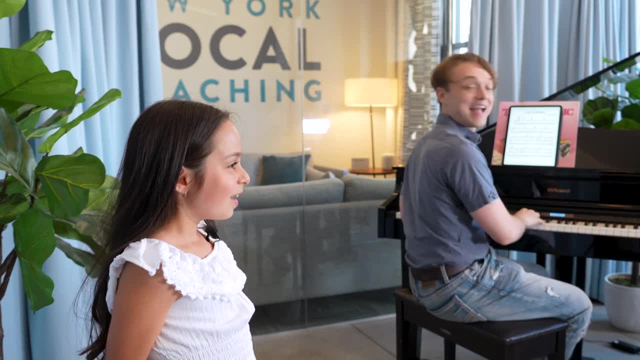 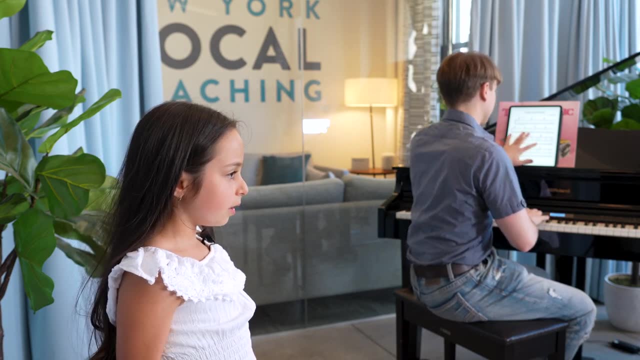 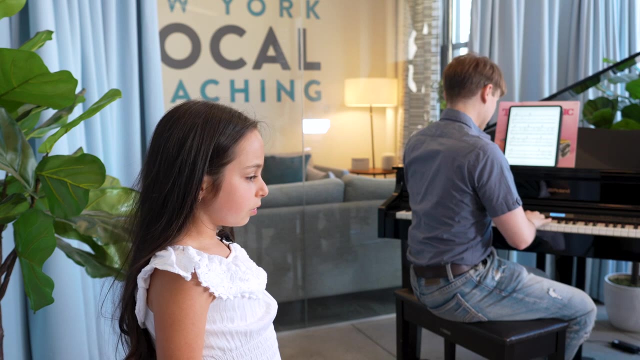 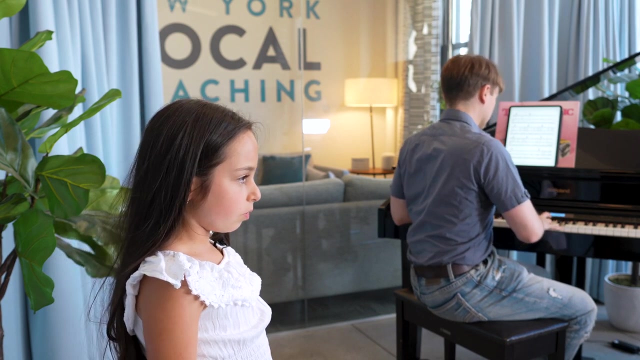 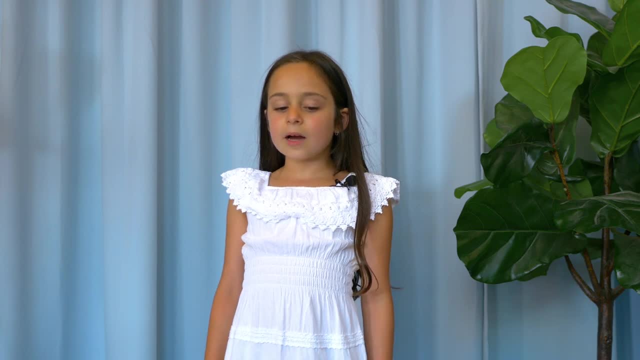 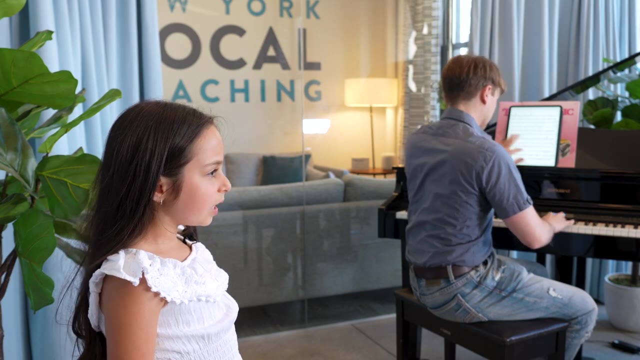 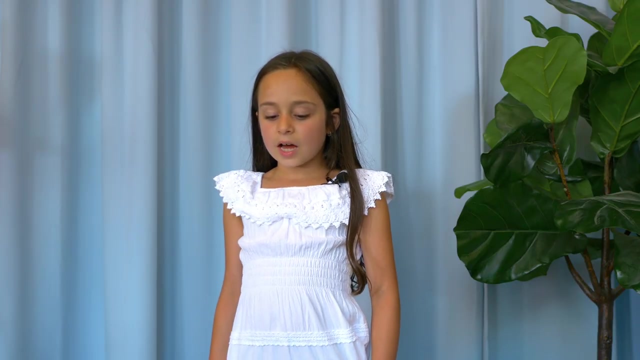 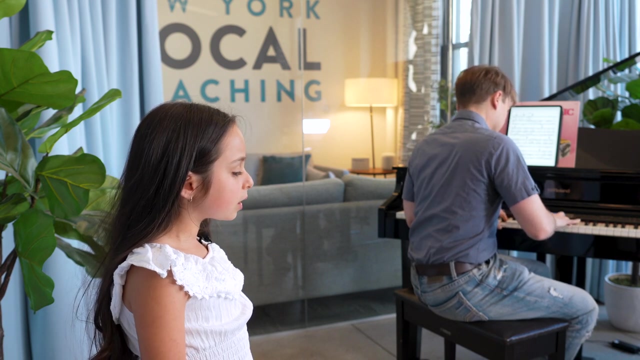 They can say. they can say: we've lost our mind, I don't care, I don't care if they call us crazy. We can live in a world that we design, Cause every night I lie in bed. The brightest colors fill my head. A million dreams are keeping me awake. 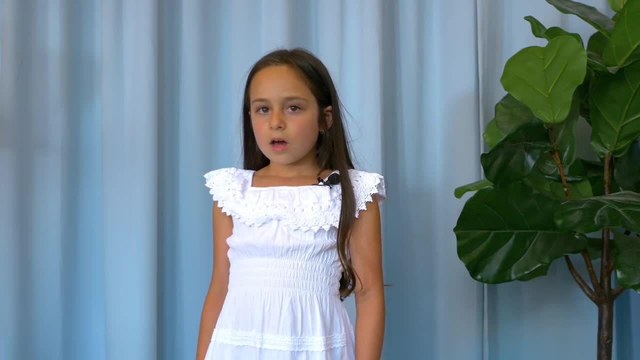 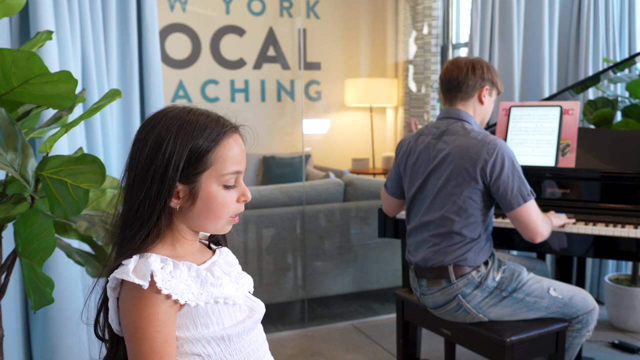 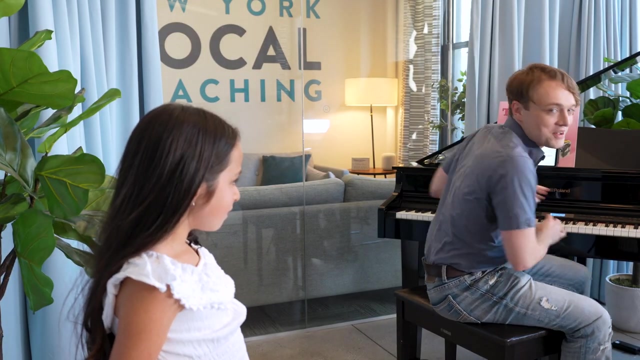 I think of what the world's gonna be, A vision of the one I see. A million dreams is all it's gonna take. Oh, a million dreams for the world we're gonna make. That was so awesome today. Join me and Emmy next time for part two.